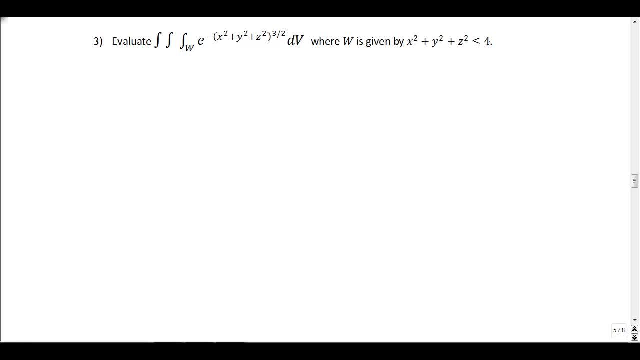 to make the choice of which one to do In this particular case. here, what I see is a couple things. I see this x squared plus y squared plus z squared, So that makes me think. well, that'd be rho squared in spherical. that's a little bit nicer than in rectangular. So let me just write. 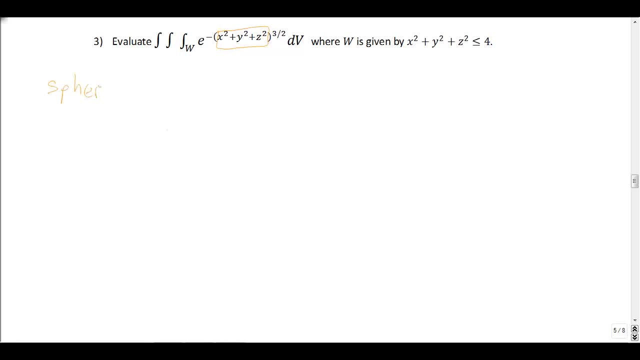 that out here is that in spherical we have x squared plus y squared plus z squared. that works out to be rho squared squared. But if you did that in cylindrical, what you get is just the x squared plus y squared is r squared. whoops, let's rewrite that whole thing again: x squared plus y squared plus z squared. 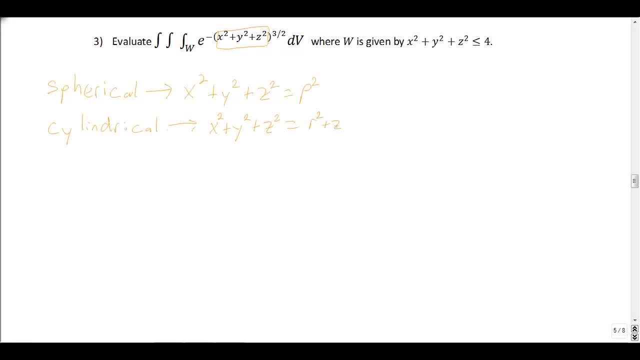 then the x squared plus y squared is r squared, and then you have the z squared left over. So if I have this x squared plus y squared, but no plus z squared, that tends to make me think cylindrical, because I have the r squared, But when you have x squared plus y squared plus z, 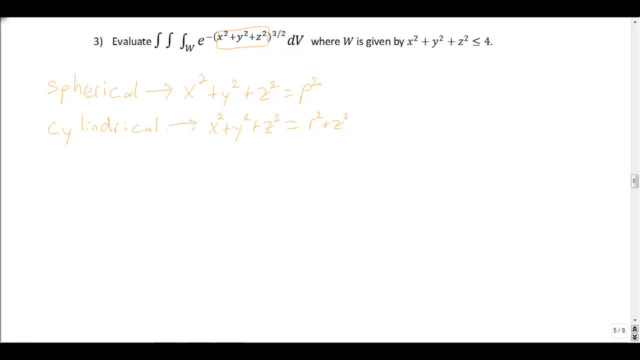 squared that tends to make me think spherical, and that's real squared. Now there's other factors that can come into play that can change you from one way or the other. One of those things is the region we're integrating over. In our case, what we have is we have another x squared plus y squared. 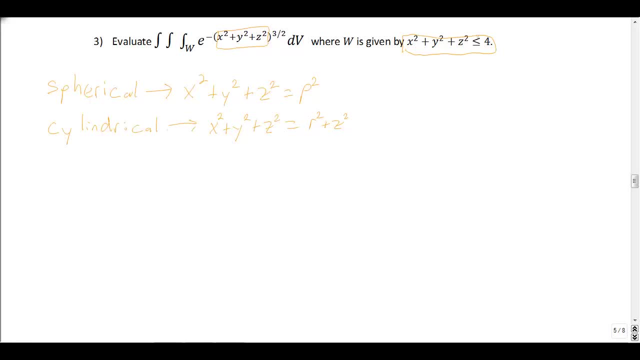 plus z squared. So our sort of outer region is really a sphere of radius two here, and because it's a sphere that makes me think spherical. but I get another x squared plus y squared plus z squared. So everything here makes me think let's do this in spherical, Okay. so let's go with that. 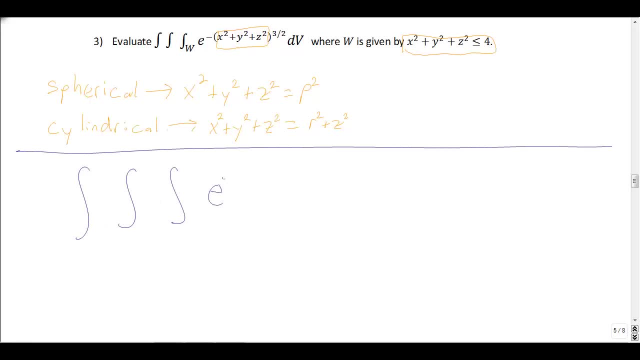 I'm going to do our bounds e to the negative. let's see x squared plus y squared plus z squared, that's rho squared. and then we take that to the three halves, which seems a little bit scary. It's actually going to work out nice. It'd be a fortunate thing that we have the three halves here. 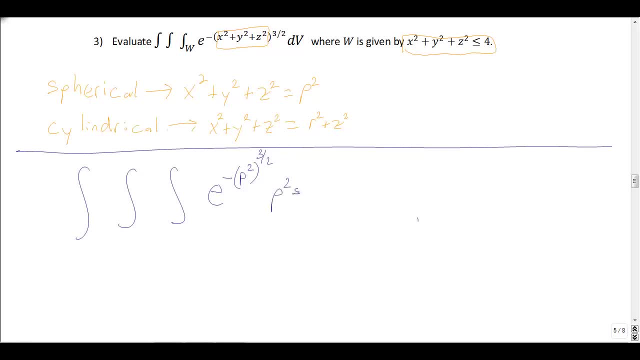 in a bit. and then we need our Jacobian, that's rho squared sine phi. and then we need to pick an order of integration. Often this is set up well for one of two reasons. One is to get our integration to work out. It's actually not going to be an issue here. The other 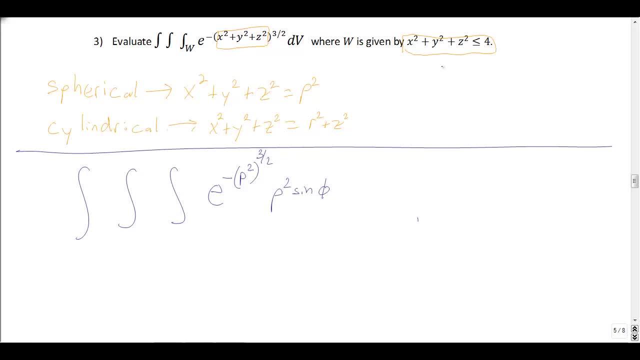 one is to fit sort of our region and get nice bounds. So here this is a sphere that's really nice in spherical coordinates. so it's going to turn out. it does not really matter what order we do these in. One thing I might do is do phi first. Here I guess I'm doing d phi d theta d rho. 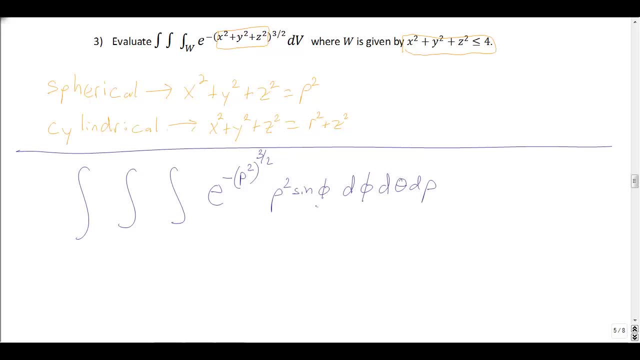 The idea of doing phi first is sometimes: these trig functions we'll integrate to zero and then sort of, you're done because you get zero and you integrate that you get zero from there now. Now, in this particular case, I can tell that I'm not going to get zero, because if I 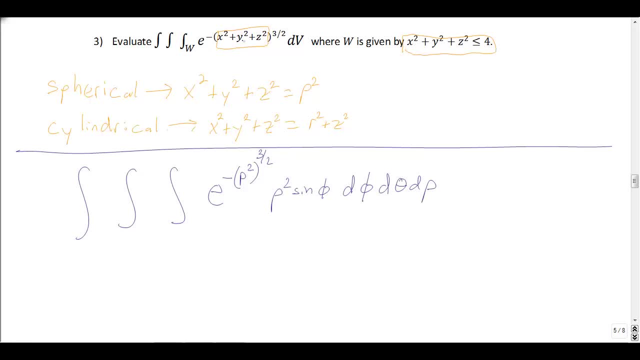 look at the integrand the function I'm integrating. it's e to something. e to anything is always going to be positive, and so I'm essentially adding up a bunch of positive. well, masses, I guess Here are a bunch of positive things, so I'm going to get a positive. 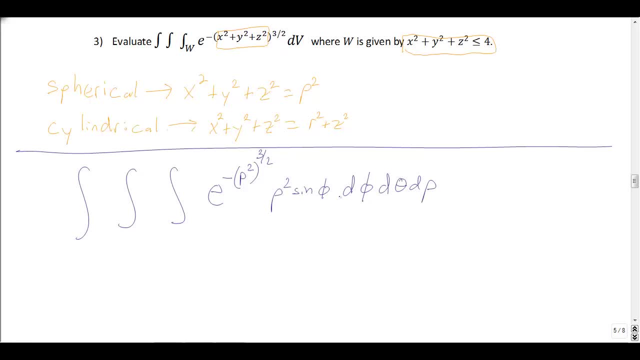 value in the end. So I know that won't happen, but sometimes it's nice to get the trig function to be zero Now. now our bounds Rho, so that starts at zero and it's going to go out to the outside of the sphere. 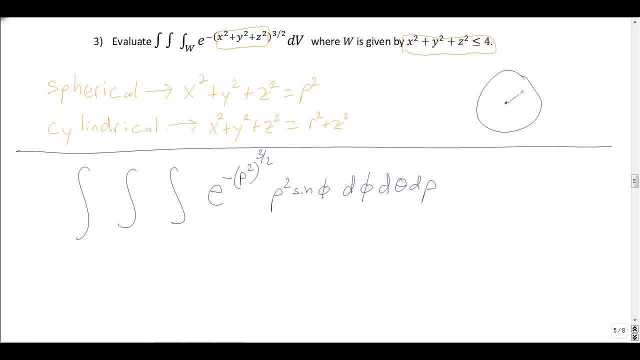 So I'm just going to draw a circle for the sphere Rho starts at zero and sort of. you just shoot out wherever you want to be and you go until you hit this outer function. but that outer function is rho equals two, So rho goes from zero to two Theta. we're going to rotate all the way around. 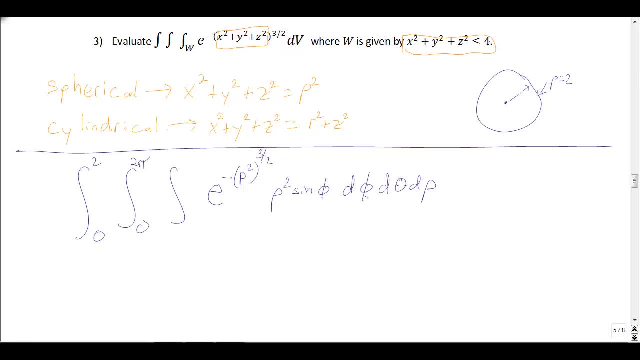 Theta goes zero to two. pi Phi phi is going to go well from the top. this is phi equals zero, and then phi sort of goes down. If we went out this way, we'd be at phi equals pi over two, so it's a 90 degree angle. 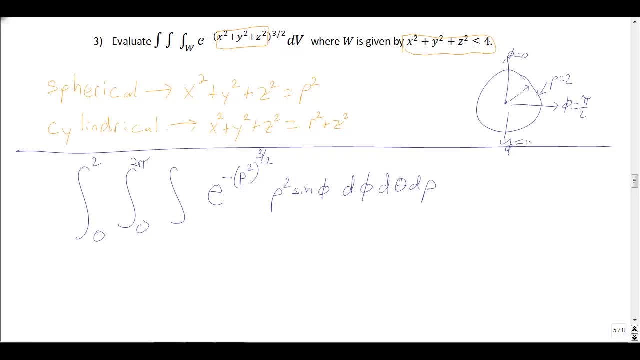 And we keep going down to the bottom That's at. phi equals pi, So pi is the largest phi will be, So we get a really nice set of bounds for a sphere here in spherical coordinates. I suppose that makes sense. What's nice about these is: all these bounds are just numbers here, so there's no like. 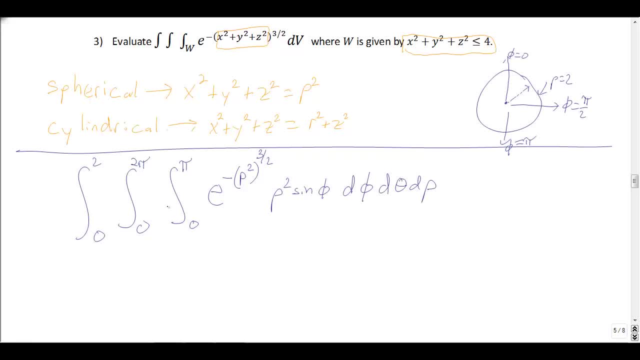 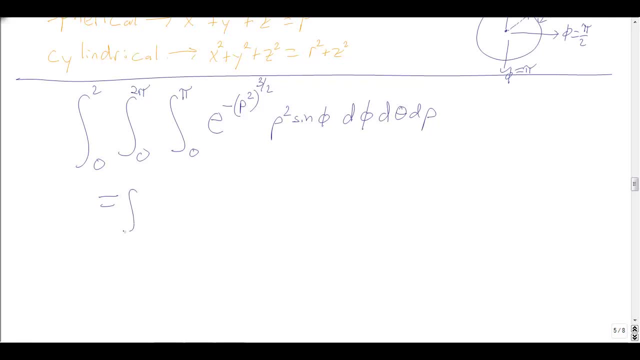 rows, or phis or thetas in the bounds. It generally makes things a little bit easier. Okay, now we just need to evaluate our integral. So the first thing I'm going to integrate is the theta. So I get zero to two. 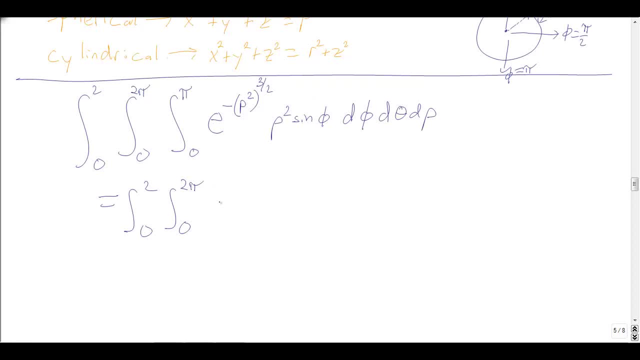 zero to two pi. I'm going to simplify this thing on the inside as I go. So e to the negative rho squared to the three halves, I'm going to multiply those exponents Whoops, and I'll get e to the negative rho cubed and I have a rho squared. 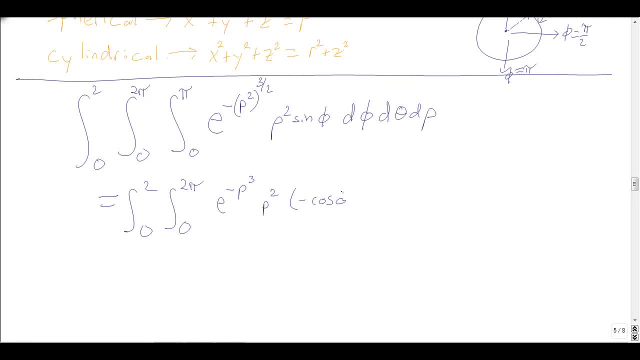 And now I'm going to integrate sine phi That integrates to negative phi, That's negative cosine phi. I'm going to evaluate that from phi equals zero up to phi equals pi, Theta, d, rho, yep, And so I get an integral zero to two. zero to two pi e to the negative, rho cubed. 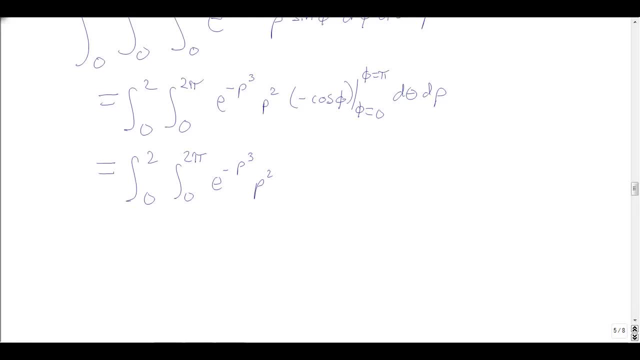 my rho squared. When I plug in pi for phi, I get negative. cosine of pi that's negative, of negative one That turns into a positive one. Cosine of pi is negative one. Cosine of zero is one. so I'm going to subtract a negative one. 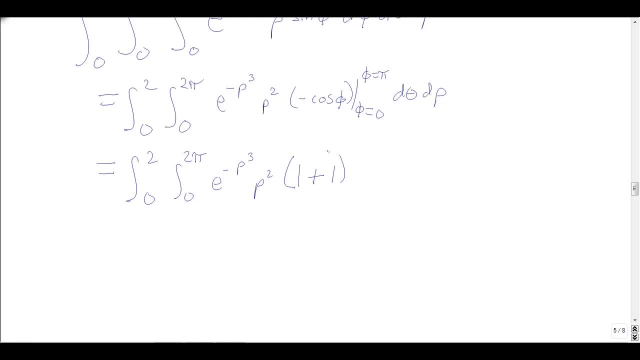 I'm going to get another plus one. So that was the thing where, if you could get the signs a little bit different, you might get a one minus one equals zero. That's why I maybe thought: oh, let's try phi first and see if something nice happens. 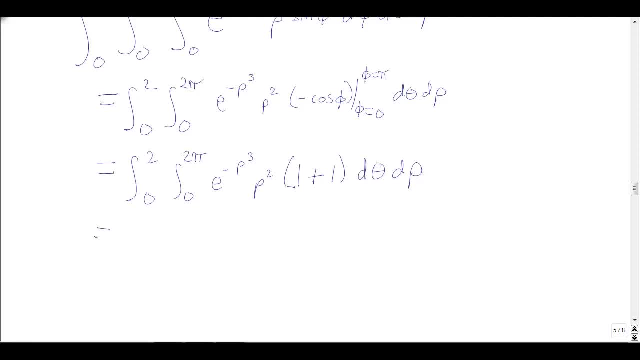 So d theta, d rho. So what I'll get, the one plus one is a two. I'm going to integrate from zero to two And then I'm looking at, I'm integrating with respect to theta, from zero to two pi, but there's no thetas here. 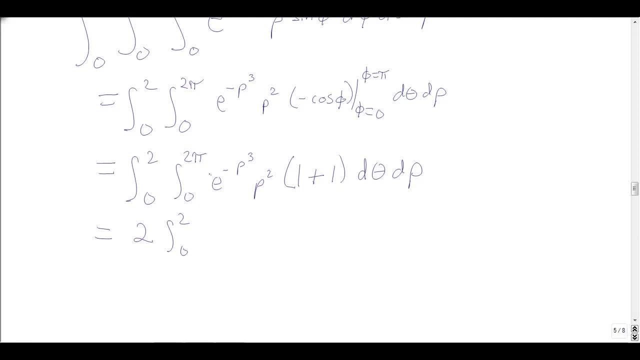 So essentially that means I'm just going to multiply. I'm going to multiply by the length of this interval, which is two pi. I'm going to pick up another two pi. I'm going to have e to the negative: rho, cubed rho, squared d rho. 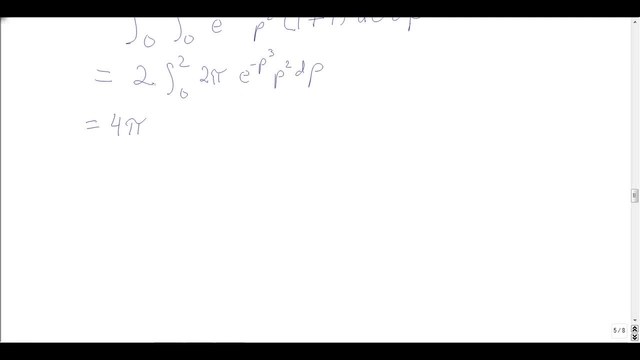 And so what I get is four pi when I do the two pi times the two, And then I need to sort of do an antiderivative. So what I'm going to do is focus on this exponent and think of u as negative. rho cubed. 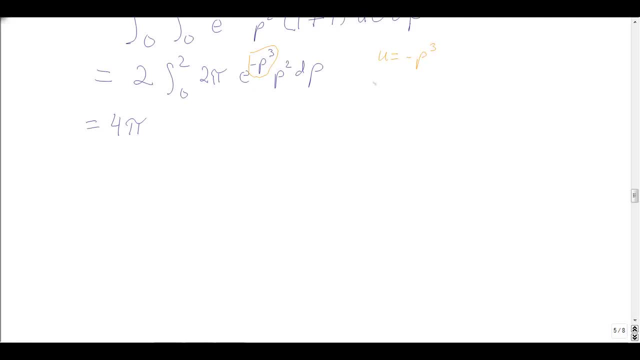 And then I have an e to the u, which would integrate to e to the u, But then I need to have du floating around. That's negative three. rho squared b? rho. Well, we've got the rho squared d rho. We're missing this negative three here. 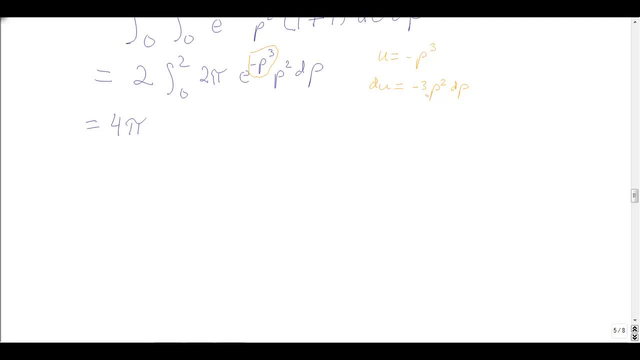 We can divide by negative three, sort of multiply and divide by negative three to take care of that. So that's no problem here And you can see this is going to just work out and give us an antiderivative of e to the negative rho cubed over negative three. 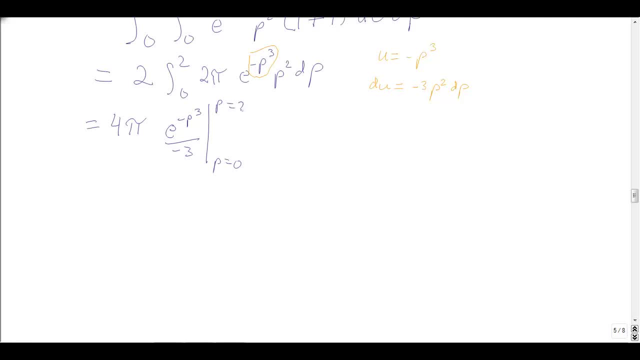 And then we're going to evaluate that from rho equals zero to rho equals two, And so what we get, let's see we have a four pi over negative three, And then we can evaluate e to the negative two. cubed is eight. 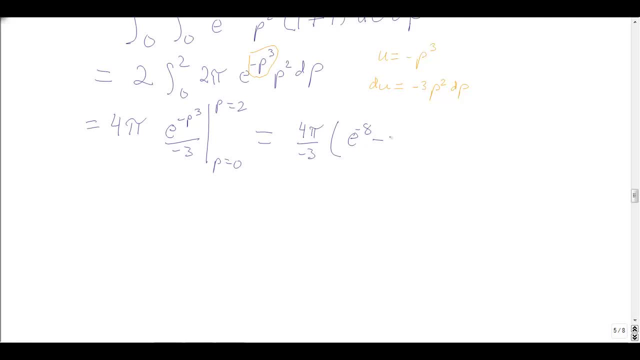 e to the negative eight. When I plug in a zero I get e to the zero, which is one, And maybe a little bit of a simplification I can do with this. I have this negative out inside. I can change the order around on this. e to the negative eight minus one. 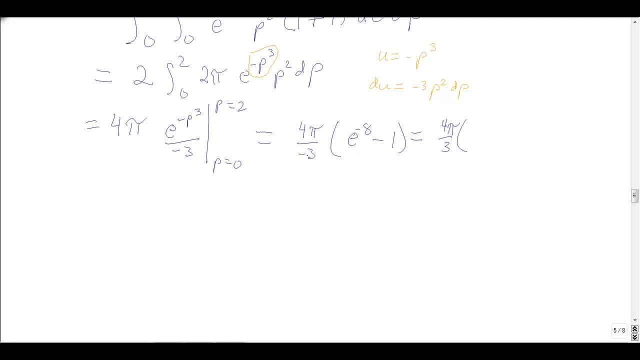 So I would tend to write this as four pi over three, Basically distribute the negative one, and then I switch the order- It's going to work out to be one minus e- to the negative eight. Now note, I said I was supposed to get a positive answer. 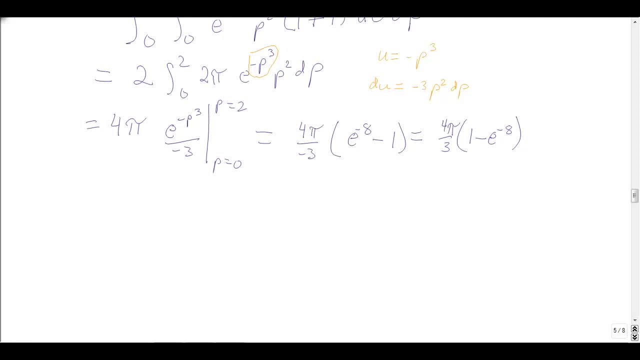 e to the negative eight is one over e to the eight. So e to the negative eight is one over e to the eight. e to the eight is going to be fairly big Here. that's like two to the eighth, well bigger than two to the. I'm sorry. 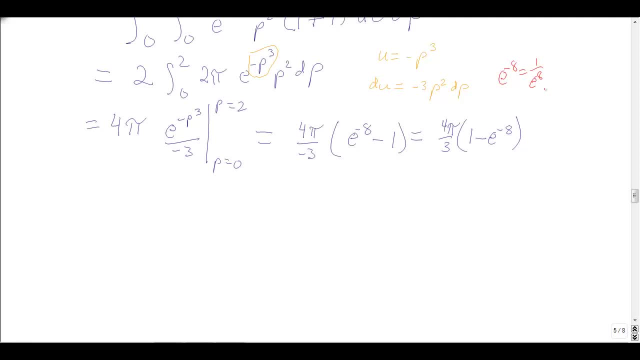 e to the eighth is bigger than two to the eighth. Two to the eighth is what, 256.. This one over e to the eighth or the e to the negative eight is going to be quite small. So this is going to be a positive. 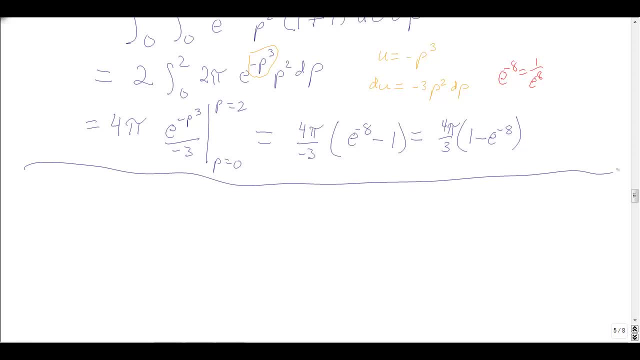 One is going to be much bigger. Okay, so that was spherical coordinates. Let's try the original integral in cylindrical. So what we're going to get is a triple integral, And then we get e to the negative. It was x squared, let's just rewrite it. 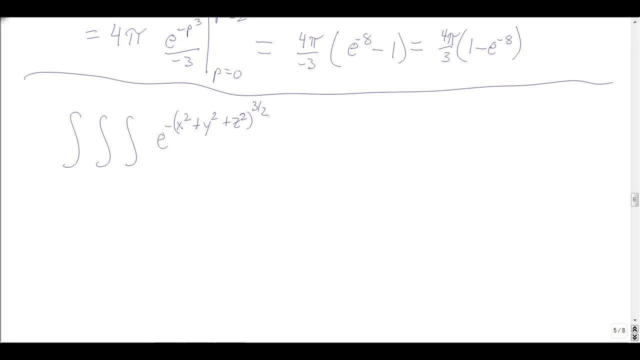 Plus y squared, plus z squared To the three halves, and then we get a dv And we're integrating over that ball here Or a sphere. So if we go to cylindrical, I'm going to get e to the negative, x squared plus y squared. 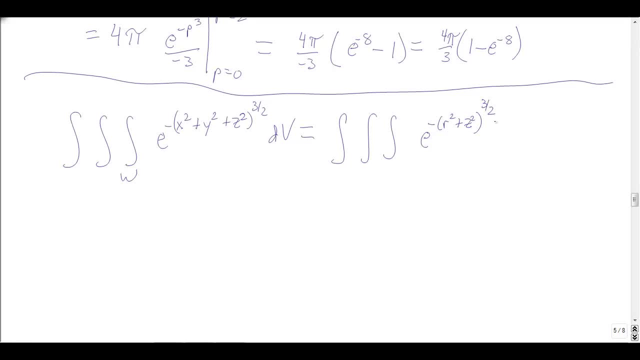 It's going to give me r squared Plus z squared to the three halves. My Jacobian for cylindrical is r, And now I have to set up some kind of order of integration here. So I'm just going to write: how about dr d theta dz here? 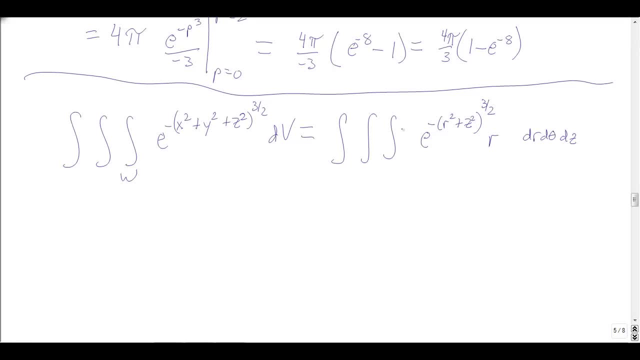 We can change these around here once we set the bounds here. But actually I'm not going to worry about that too much because I'm going to have trouble integrating these. So, theta, I can integrate this theta here, Because there's no theta here. that's just going to be a multiply by.